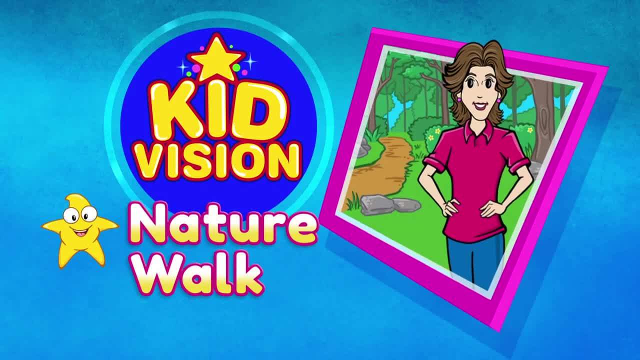 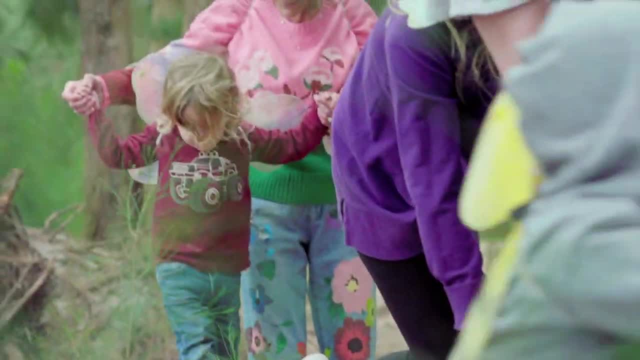 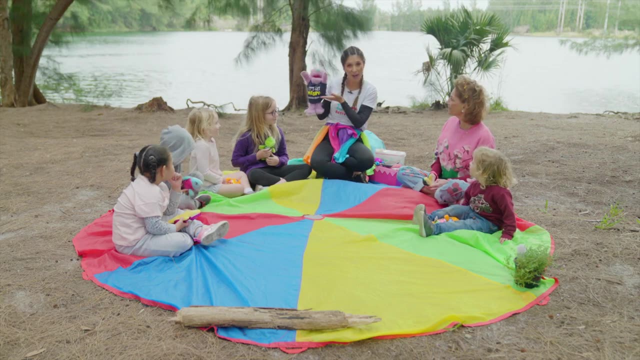 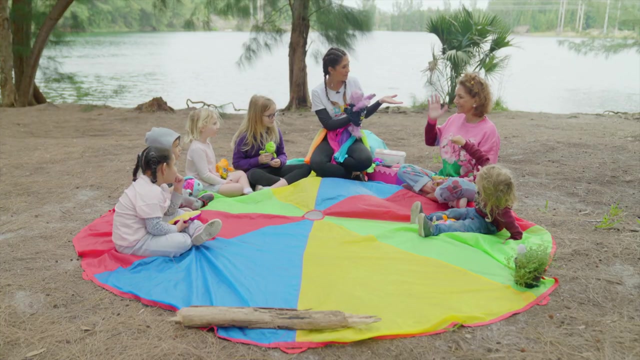 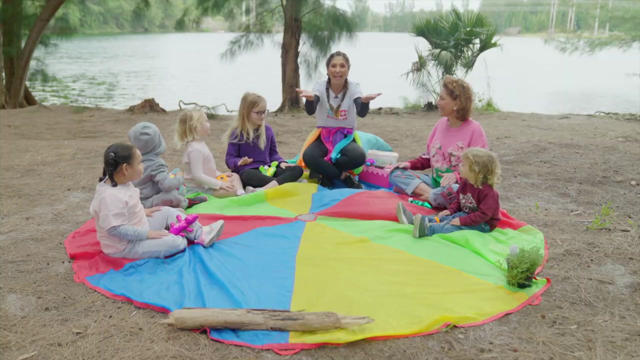 Hi, my name is Ms Alexa and this is my friend, Fred, And today we're going to do nature class and we have a very special guest. We have Ms Penny here with us. Hello, Can you say, hi, Ms Penny, Hi Ms Penny, Hi Ms Penny And hello friends. Hi, Today we're going 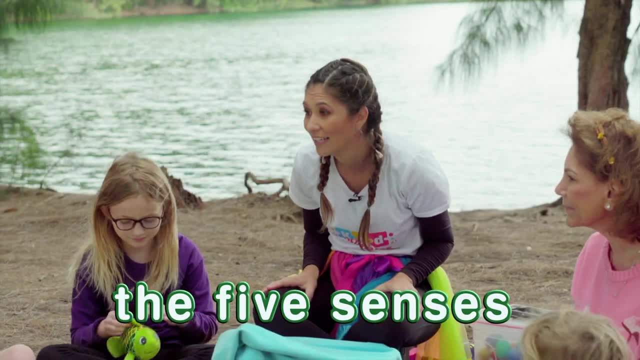 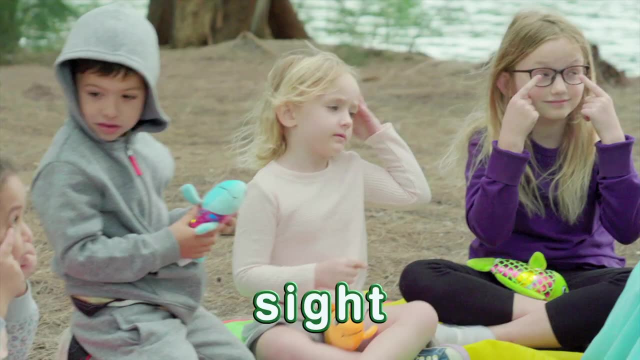 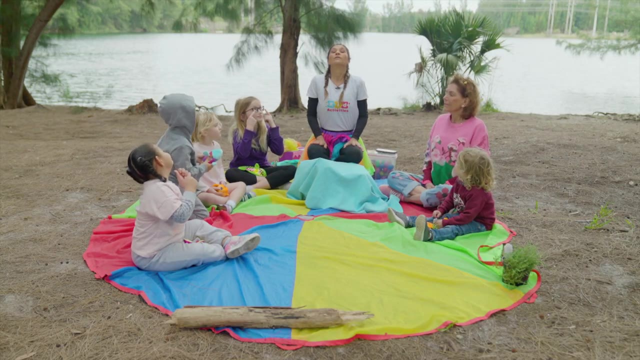 to talk about our senses. Do you know what our senses are? Yeah, Senses is how we get information from the environment. We can use the sense of sight. Go like this: Open and close your eyes. We use our eyes to see things. Go like this: We use our nose to smell. 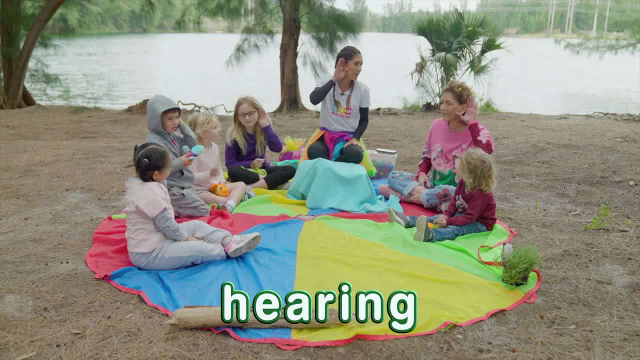 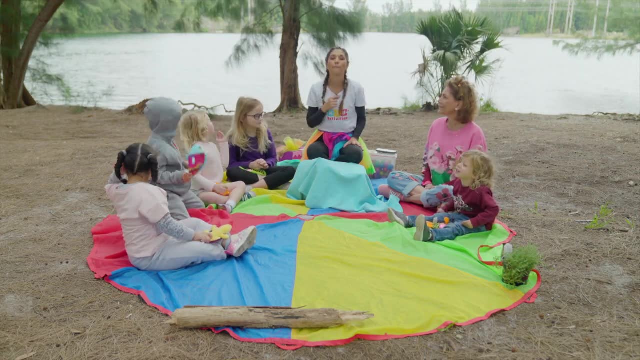 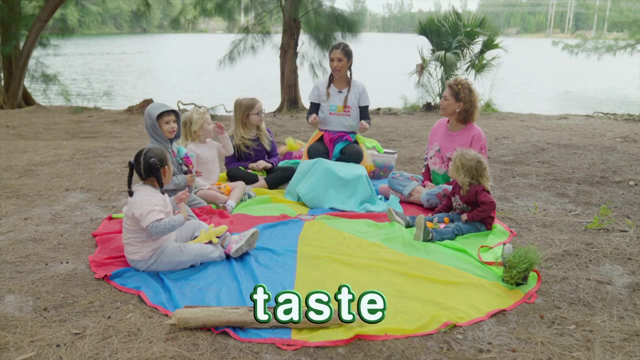 Like this. What do you hear? I hear a woodpecker. We use our ears to listen. Go like this. We use our tongue to taste. And what's this? Wiggly fingers, wiggly fingers. We use our. 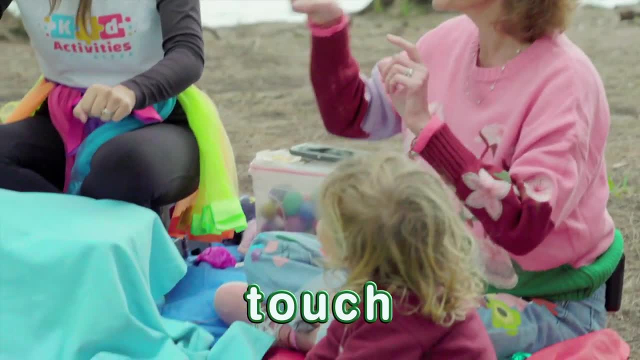 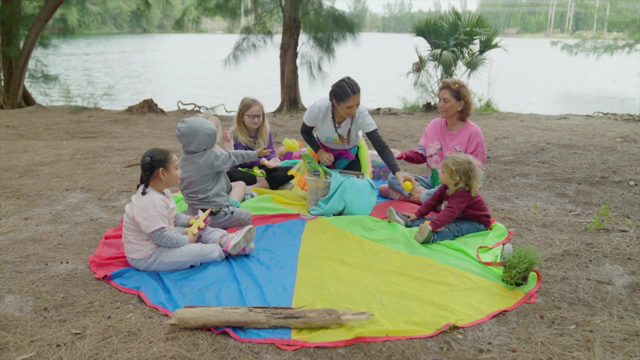 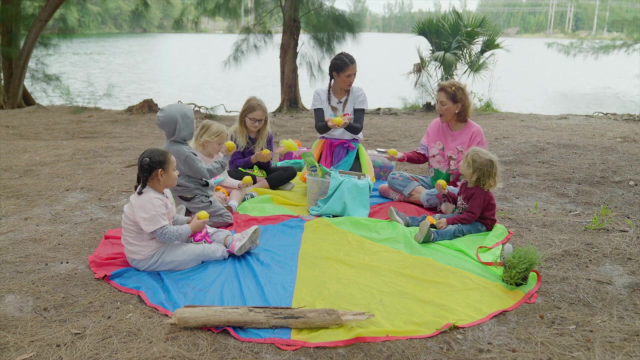 hands to touch. Good job, Everybody. close your eyes and hold out your hand. Take out your hands And I'm going to give you something for you to touch. No peeking. Open your eyes. Did you know What? It's? a lemon? It's a lemon. Okay, Scratch it like this. Scratch it with. 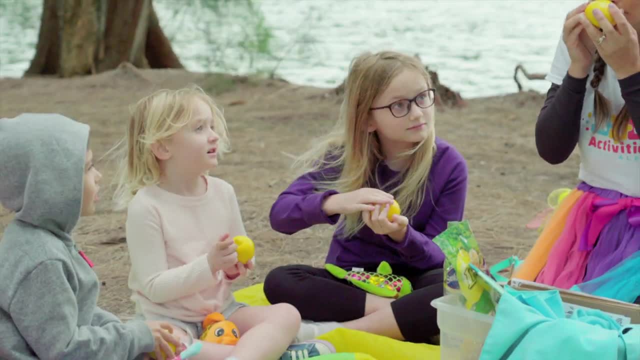 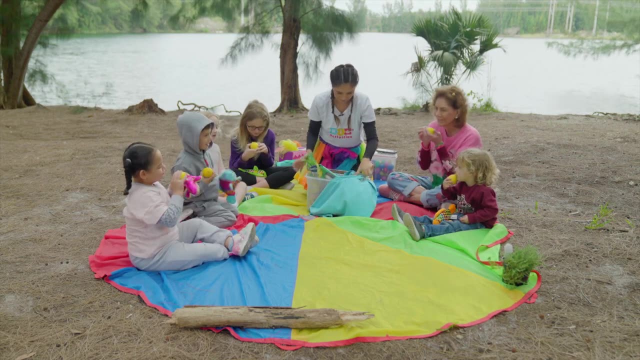 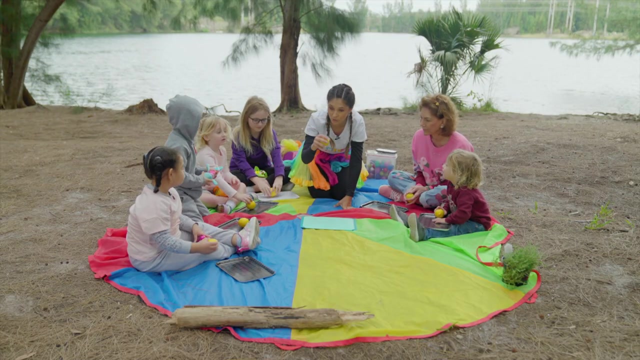 your nail, Okay, And go like this: Smell sour, like sour, because you know that lemons are sour. Yeah, Let's put my box down. Let's put my box behind. I'm going to give you a trick. Are you making sounds? Let me. 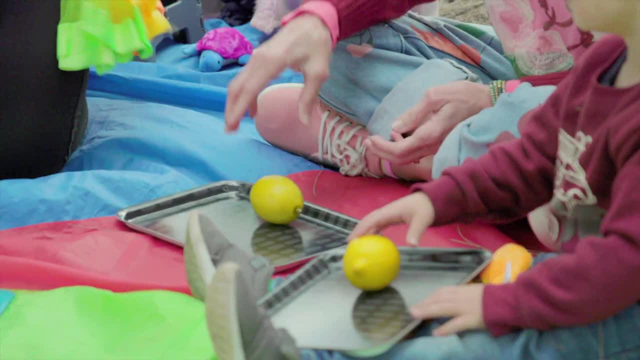 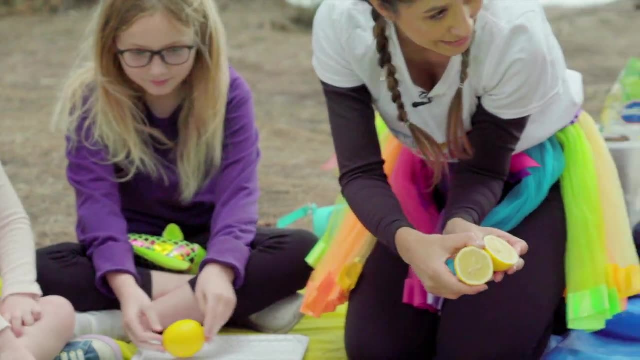 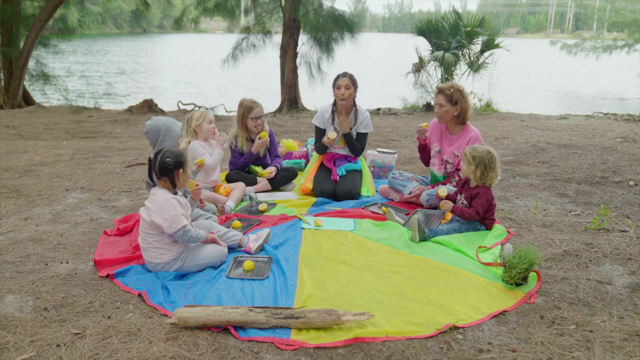 hear it? Oh, good job, I do hear. Look what I'm going to do. What do you see? Seeds, Seeds, Did you taste it? Get your tongue out And now flip your lemon like this: Oh, that's. 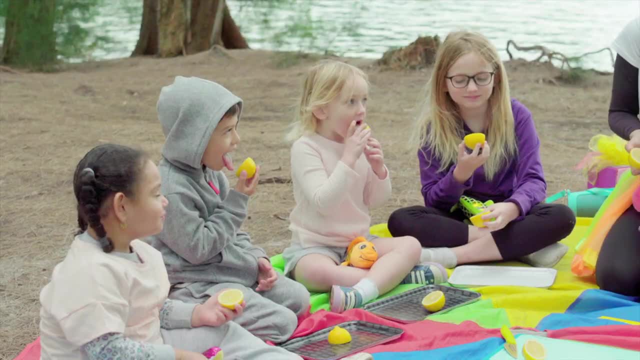 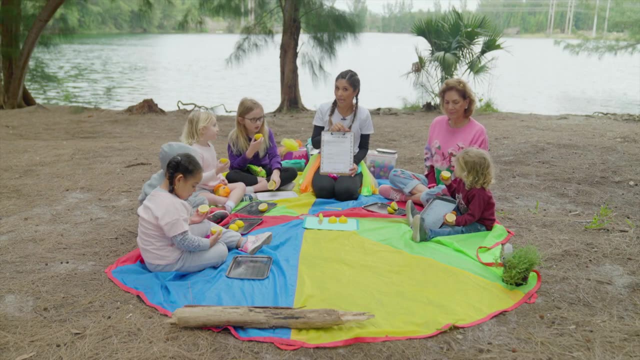 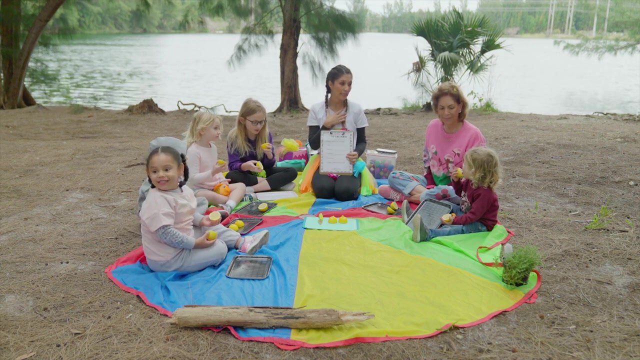 good, sour. So today we're gonna go on a nature walk and we're going to see what we find. Let's try not to eat anything that we find, because sometimes we don't know if it's poisonous. So before you touch something, please ask Miss Alexa, okay, and 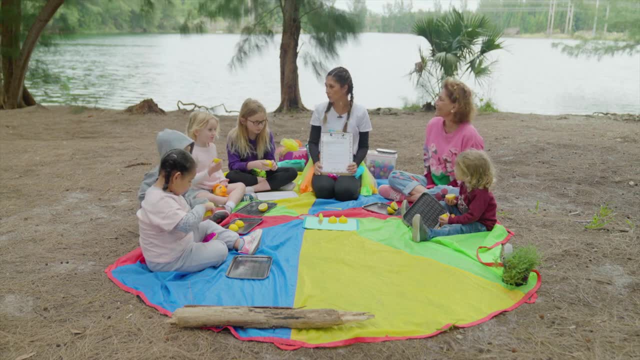 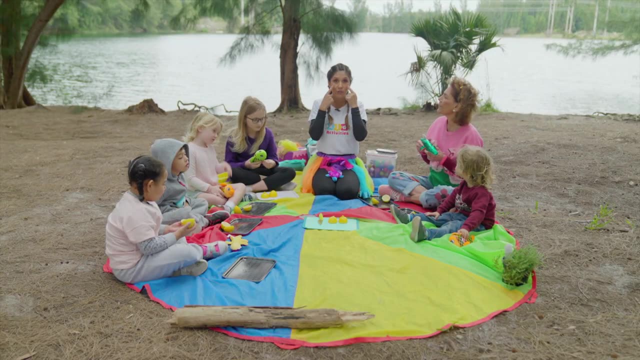 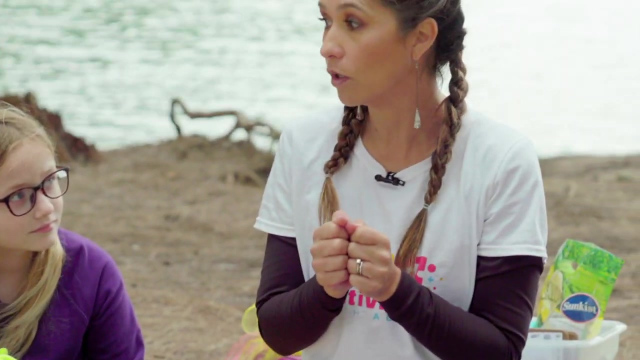 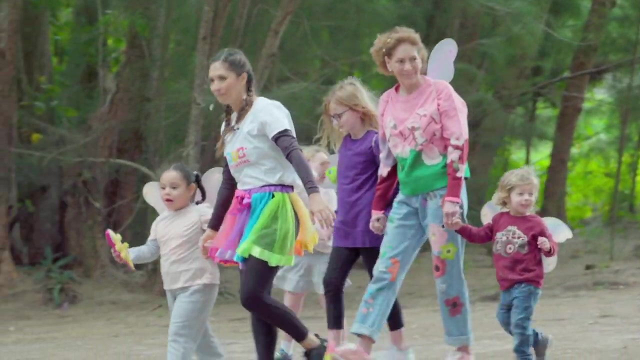 we'll observe together around the lake and things we find. We're going to do some observations. You know what observation means? It means we are going to look with our eyes, we are going to ask questions and we are going to use our nature tools to see what things. are You ready for a nature walk? Yeah, Let's go. 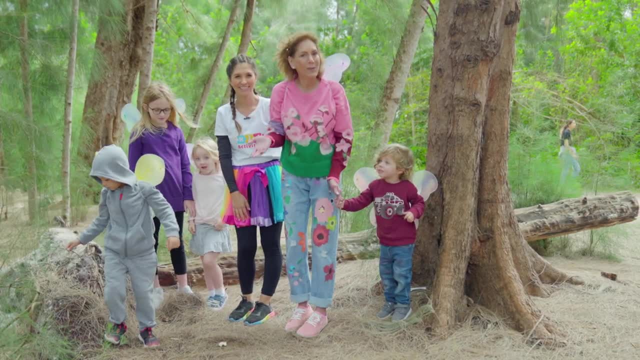 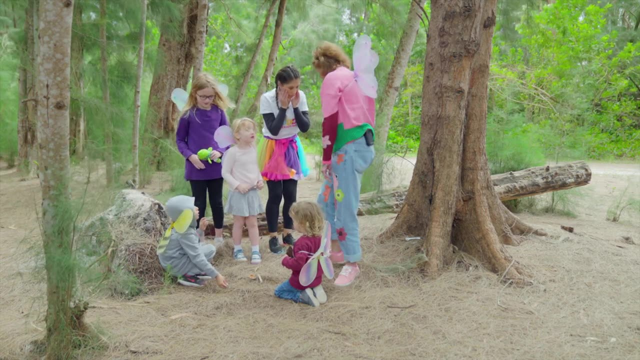 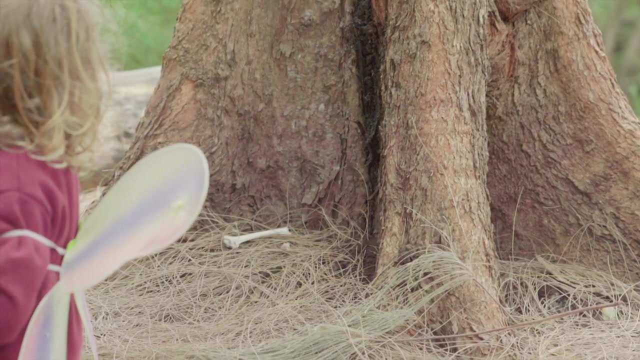 This is the first spot that we get to observe and use our senses to see what we can find. Miss Penny, look what you have behind you: Bones, Oh my goodness. Great observation, Manuel. Those are bones. KidVision, kids, we found something. but before we're going to do, 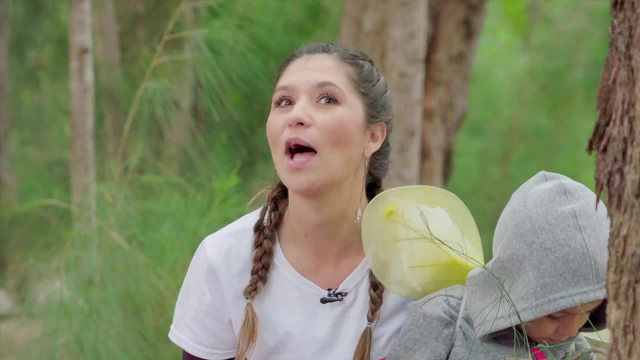 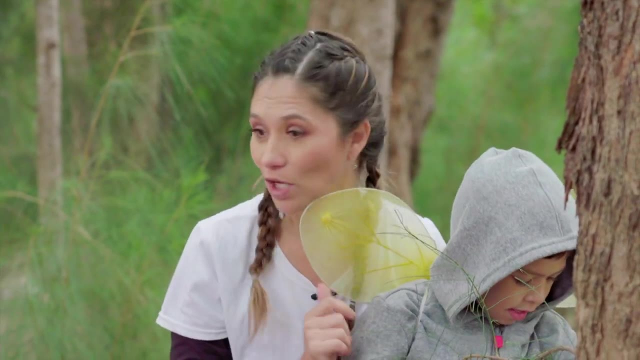 some observation. we need to keep it safe, so I'm going to tell you a little bit of the rules that we have for today, So we don't touch anything with our hands. I have tools, So the first thing that we're going to do is I'm going to give you some magnifying glasses. 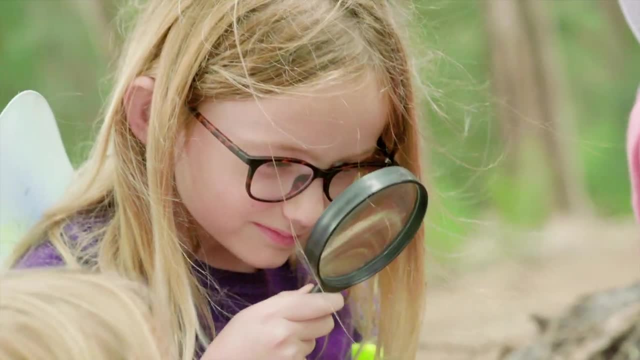 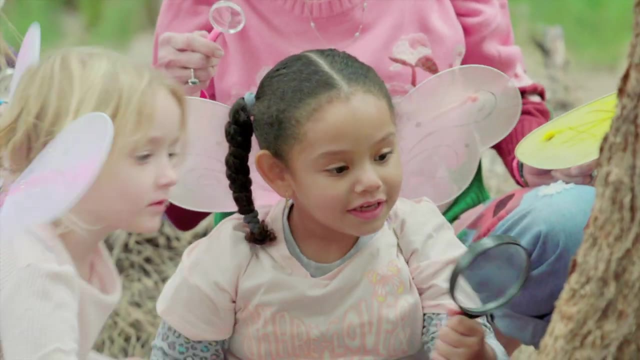 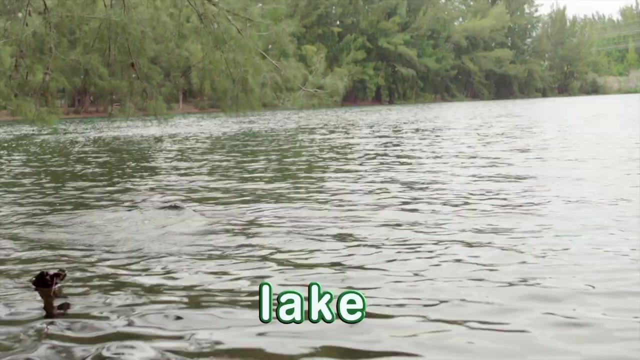 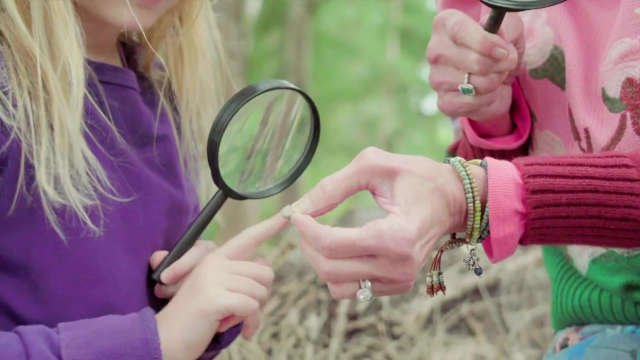 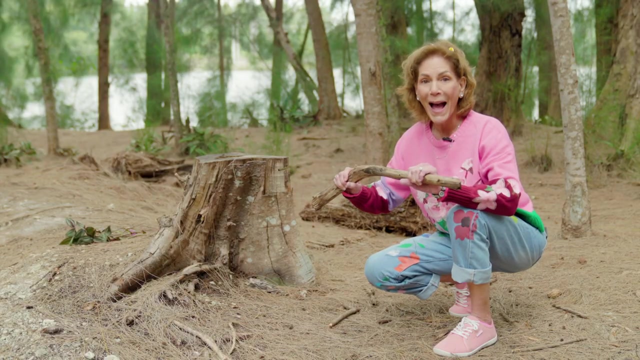 so that we can observe what we find. You see bones. What color do you see? are these bones? White, White? Who lives in this lake that could have bones- Dogs. Wow, KidVision kids. look what I found on the nature walk. 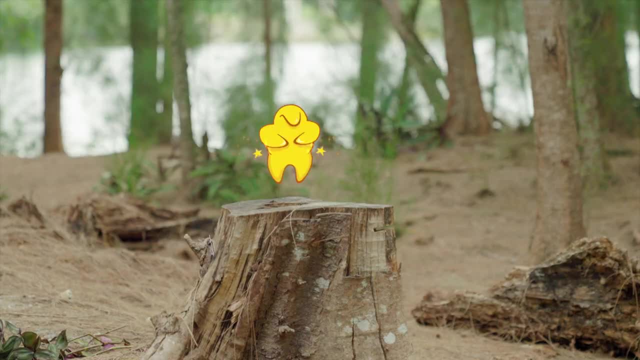 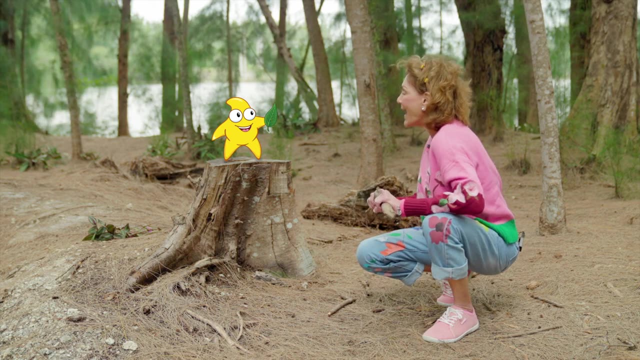 What do you think you could find on a nature walk? Oh hi, Shiny, Did you find something cool on the nature walk? Wow, that's an awesome leaf, Shiny. What else can we find on a nature walk? Wow? 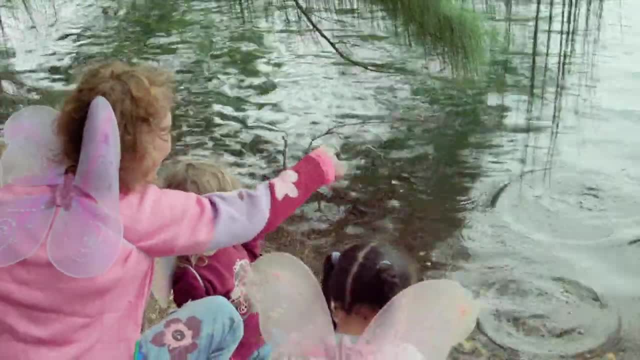 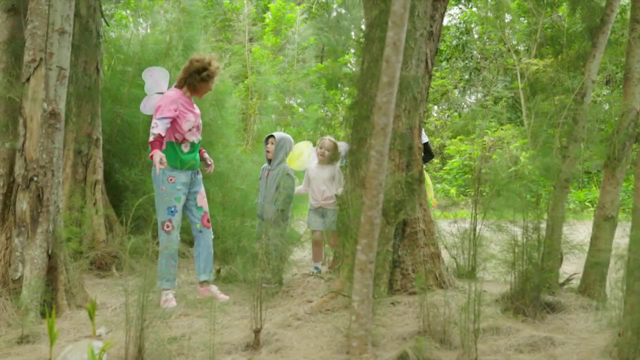 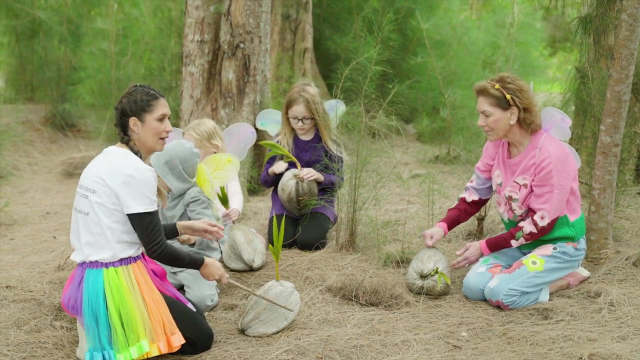 Did you find something cool on the nature walk? What else can we find on the nature walk? Wow, that's cool, It's a coconut. Do we make sounds? Yeah, it makes a sound when we tap it. Yeah, The sense of smell. 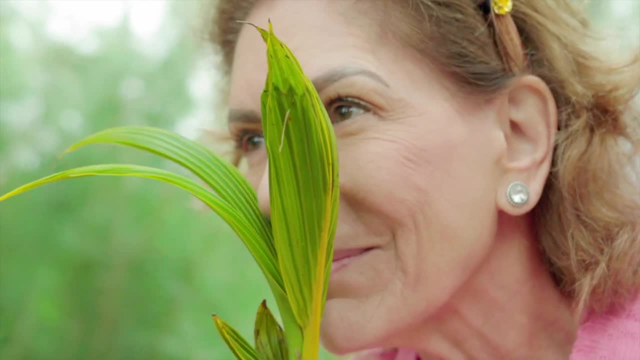 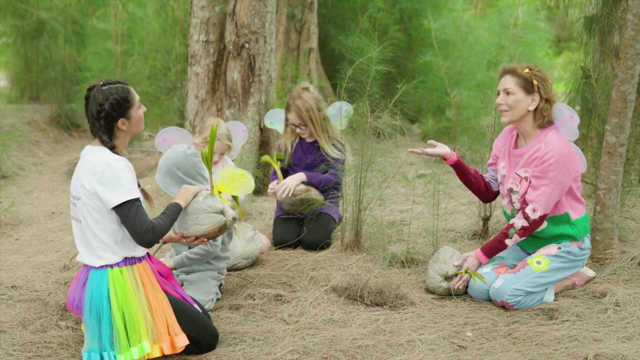 Let's smell it, Mm coconut, The sense of taste? No, just kidding, We're not going to take it. There's coconut juice that we can drink, That is true. Before it stems out, we can drink the coconut juice. 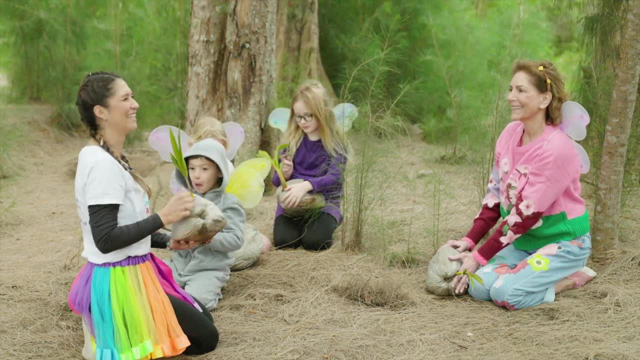 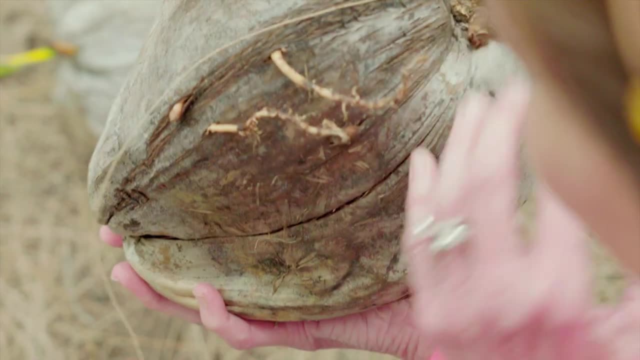 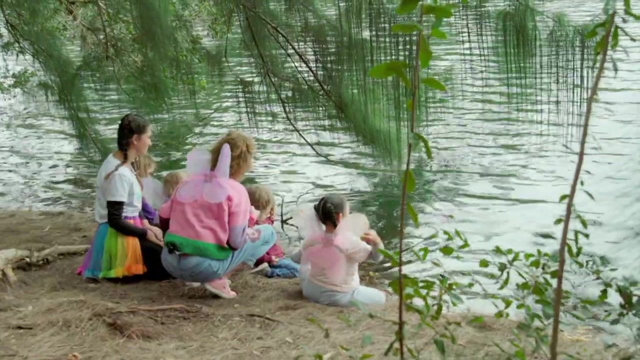 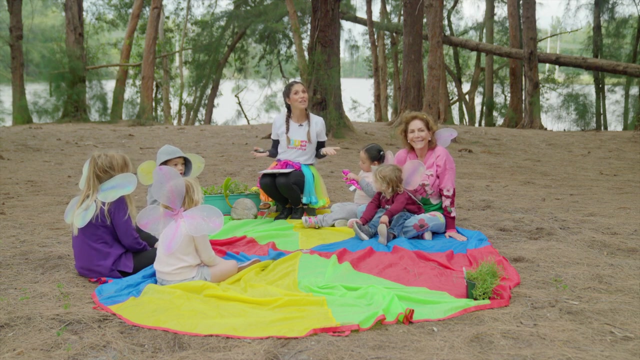 That's a great observation, Miss Penny. Thank you, Good job. Then the sense of sight. Look at the stem is growing out and the roots It is rooting. This is going to turn into a very big coconut tree. Hey, KidVision kids, We finished our nature walk and we saw so many good things. 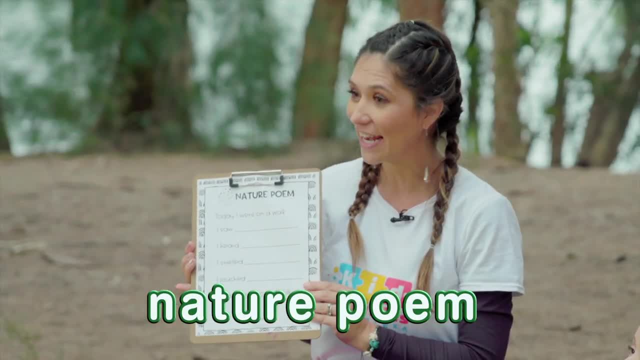 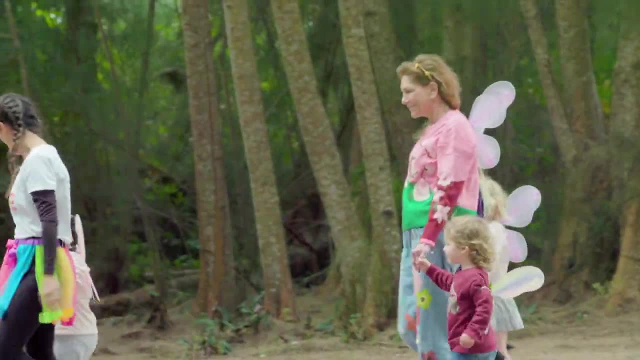 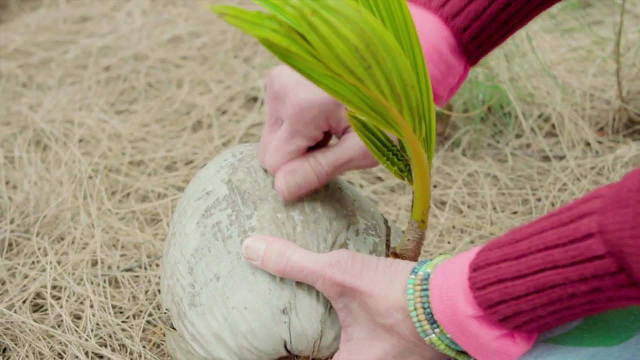 Now it is time to do our nature poem. Are you ready? Yes, Wow, Yes. This poem says: today I went on a nature walk. I saw with my eyes, I heard with my ears, I smelled with my nose. I smelled with my nose. 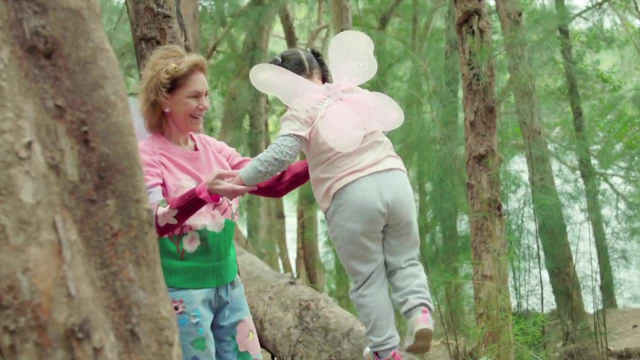 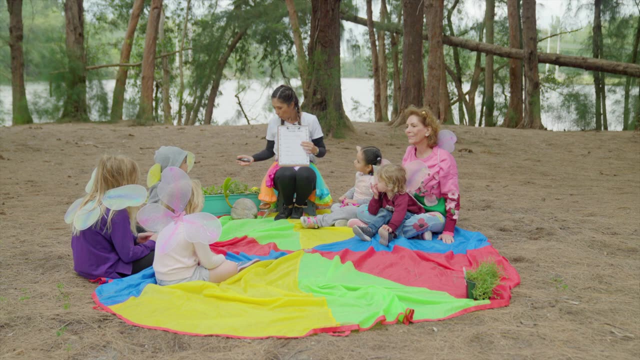 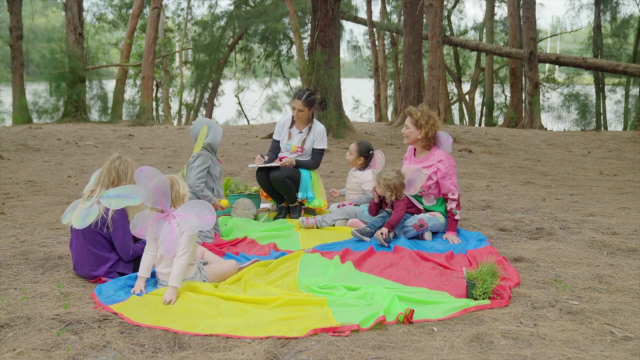 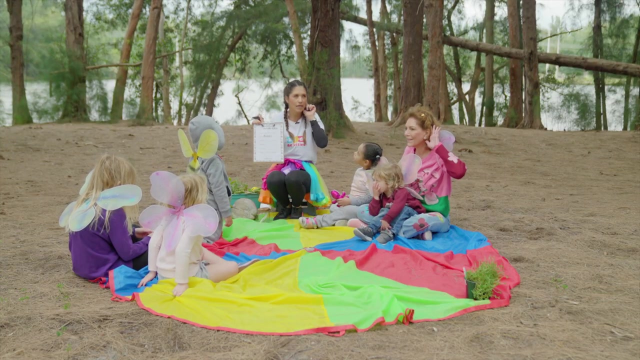 I smelled with my nose, I touched with my hands. Today I went on a nature walk. Okay, Today I went on a nature walk. I saw: What did we see? Bones, Bones- I'm going to write bones. I heard, What did we hear? 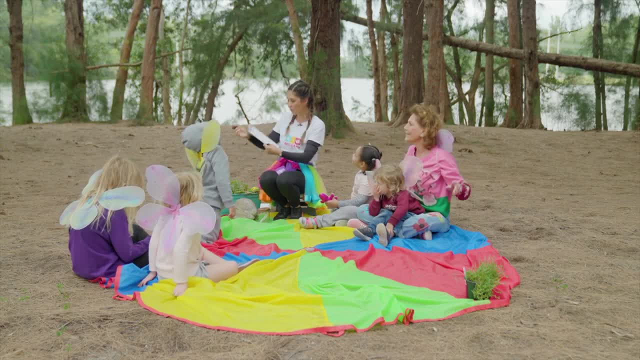 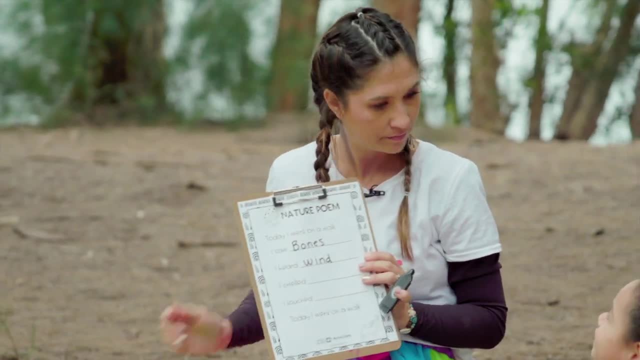 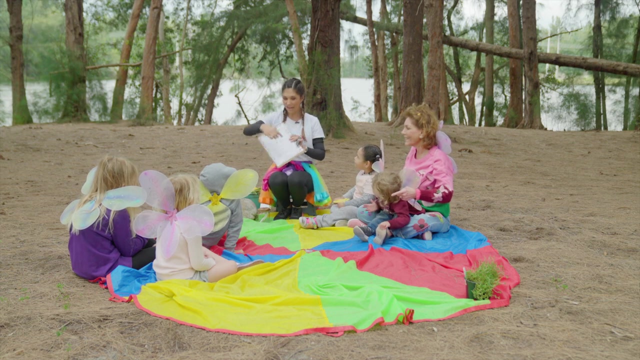 A windy, The wind when the trees were moving, The wind, The wind, I smelled, I smelled. Do we remember what we smelled? Lemon. We smelled the lemon. You're right, You're holding the lemon. I touched. What did we touch?